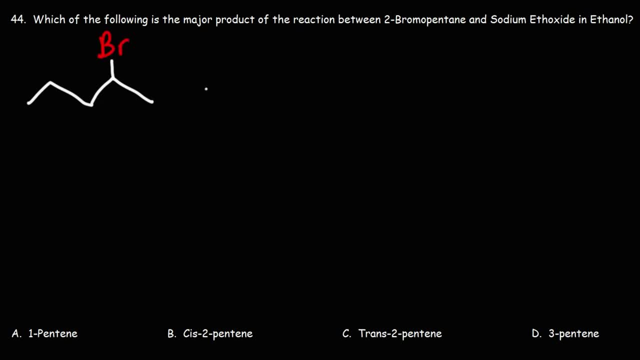 Now we're going to react this with sodium ethoxide N-A-O-E-T. E-T stands for etho And this is going to be in ethanol E-T-O-H. Now, looking at our products, we see that we're converting an alkyl halide into an alkene. 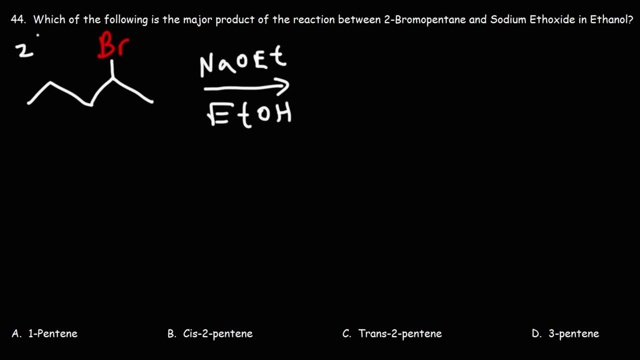 So this is going to be an elimination reaction And we have a secondary alkyl. halide Ethoxide is not a weak base, but it's a strong base. Whenever you see oxygen with a negative charge that's not stabilized by resonance, you're dealing with a strong base. 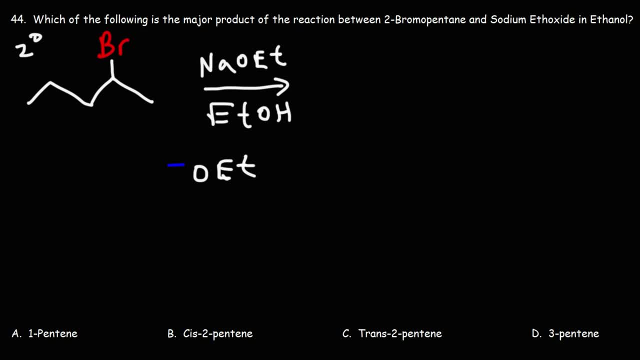 Strong bases favor E2 reactions. Weak bases favor E1 reactions. Now, on the primary carbon, we have three different hydrogens that we can take out. On this carbon, we can remove two different hydrogens. Now which hydrogen will the ethoxide go for? 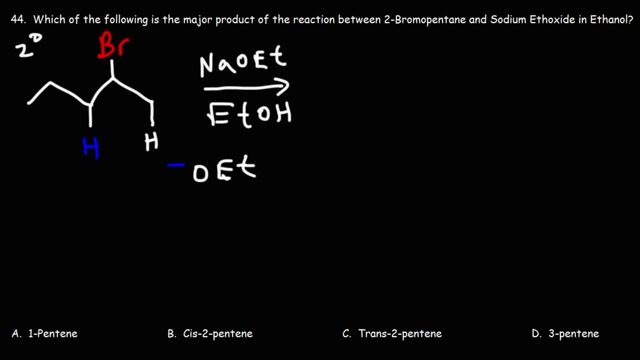 The white hydrogen or the blue hydrogen. What would you say? If ethoxide goes for the white hydrogen, the base is going to grab the hydrogen. the carbon-hydrogen bond will break. those electrons will be used to form a pi bond. 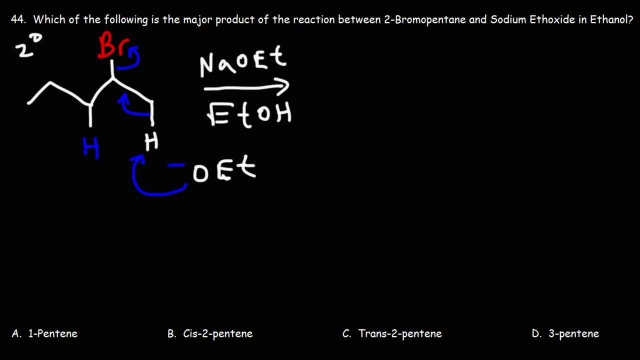 and the leaving group is going to leave. All of these processes will occur at the same time, which means that the E2 reaction is a concerted reaction mechanism. So if we go for, if the strong base removes the white hydrogen, we'll get one pentene as a product. 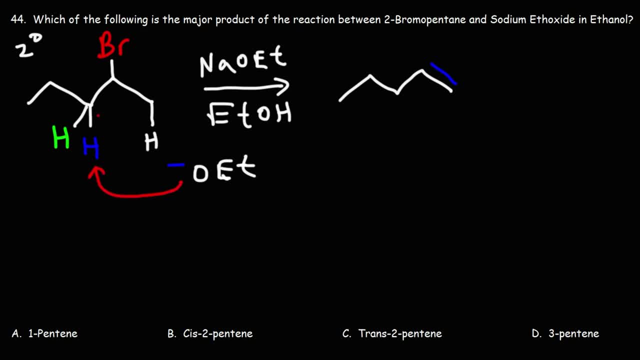 Now, if it goes for the blue hydrogen, we're going to get two pentene. Now it can go for the blue hydrogen or the green hydrogen, So we can get a mixture of products here, Depending on which one it goes for. 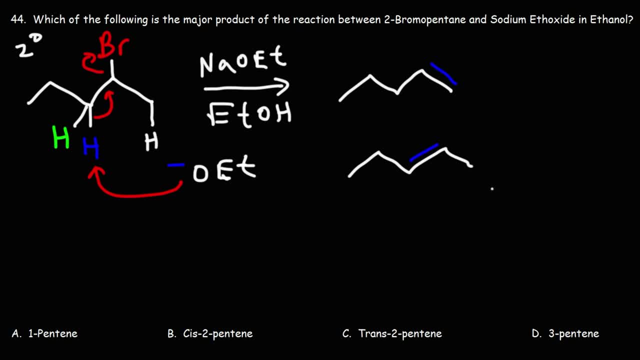 we can get trans-2-pentene or we can get cis-2-pentene. It's not possible to get 3-pentene, Because when you name this alkene, it's going to be between carbons 2 and 3,. 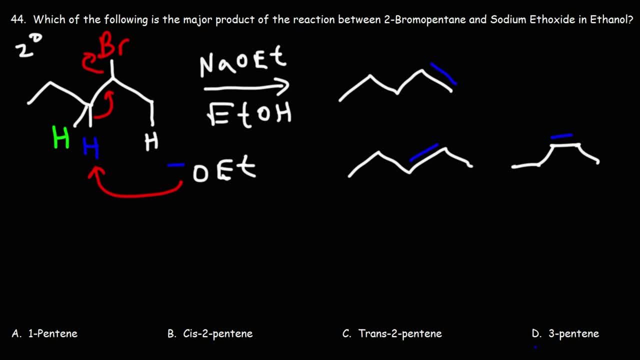 and automatically it's going to be called 2-pentene, So 3-pentene simply doesn't exist. So those are the three possible products that we can get. Which one is going to be the major product? The major product is usually the most stable alkene. 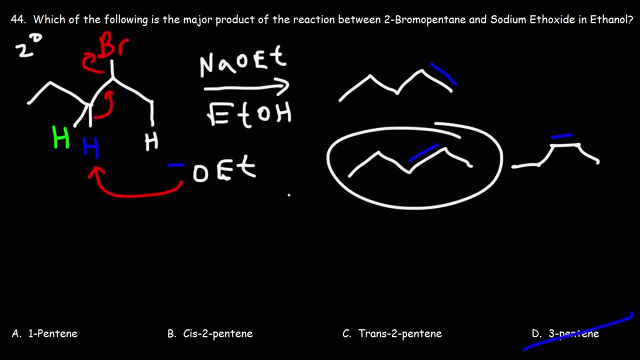 and the most stable alkene is going to be trans-2-pentene. This is a mono-substituted alkene. As you can see, if you look at the two double bonded carbon atoms, there's only one R group or one carbon. 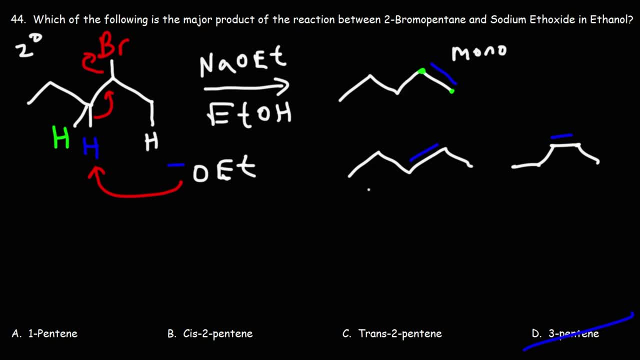 attached to those two double bonded carbon atoms. Both of these are disubstituted alkenes, So they're much more stable than a mono-substituted alkene. This one has two R groups, And the same is true for this one. 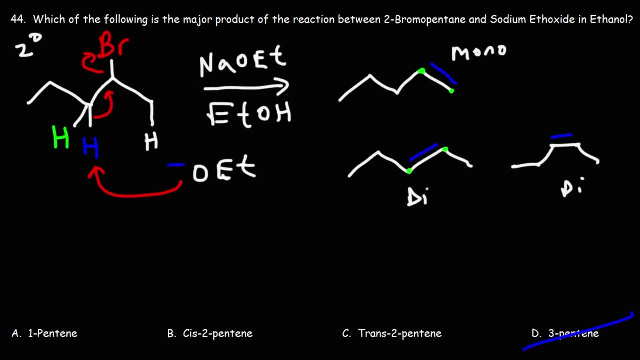 It has two R groups as well. Now the trans-isomer is going to be more stable than the cis-isomer, So that's why this is going to be the major product. The minor product, the less-substituted alkene- this is known as the Hoffmann product. 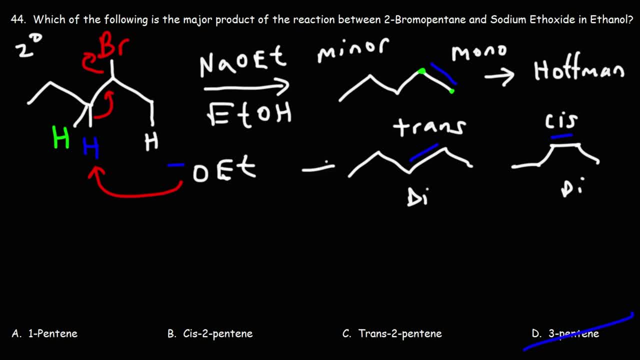 The major product, which is not always, but typically the more-substituted alkene, that's the Zaitsev product. Some books spell Zaitsev the other way, as S-A-Y-T-Z-E-F, something like that. 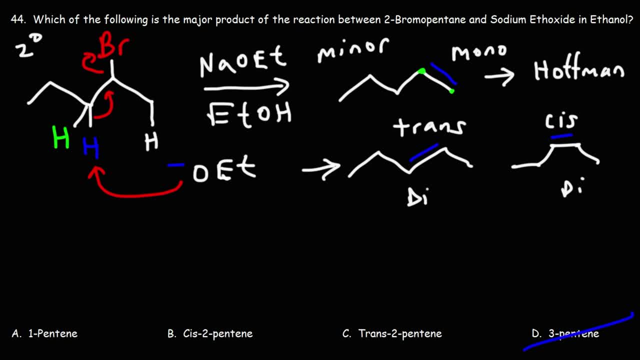 But the answer for this problem is going to be trans-2-pentene, So answer choice C is the correct answer. If you use a strong unhindered base, the major product is going to be the Zaitsev product. If you use a bulky base, 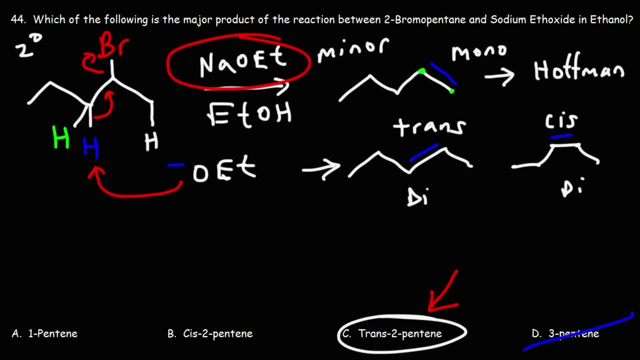 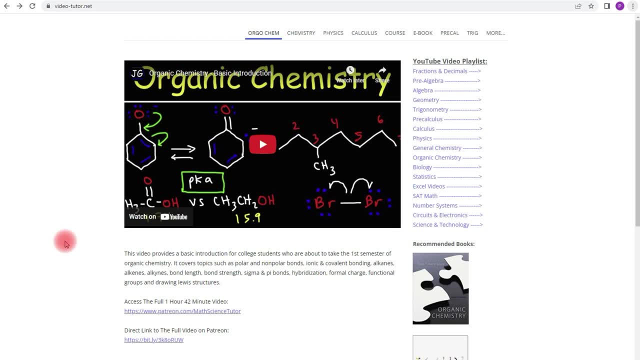 a strong hindered bulky base, typically the Hoffmann product will be the major product. Now this is for those of you who want to get access to all of my video playlists and exam review videos all in one spot. So if you go to video-trudanet-